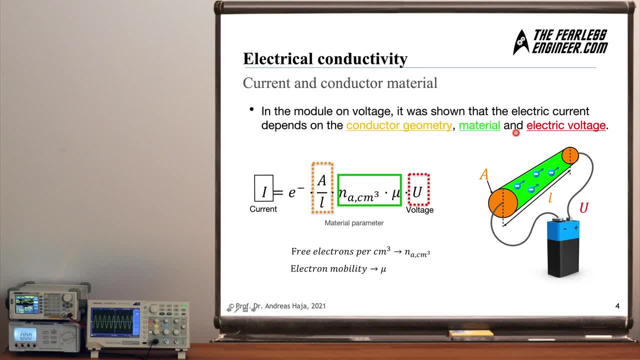 current in which the relative current DNA in a particle is measured to wake up a current, The energy of the electric current and thus the conductor parameter dividend. Either this is subject to conductor material and also the electric voltage which we apply to the poles or the terminals. 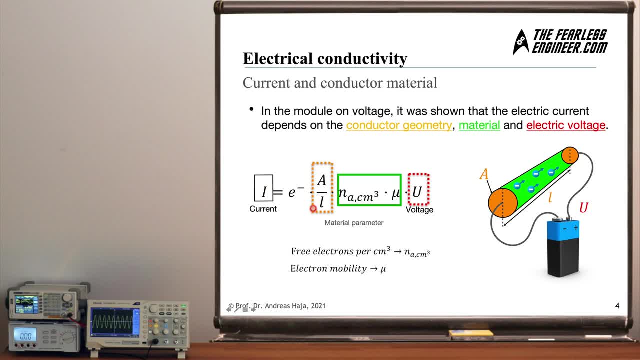 of the respective conductor, And we also came up with this formula here. If you do not know where this formula comes from, I recommend that you watch the associated videos where we talk about the electric current in order to understand how we can arrive at this definition of the electric 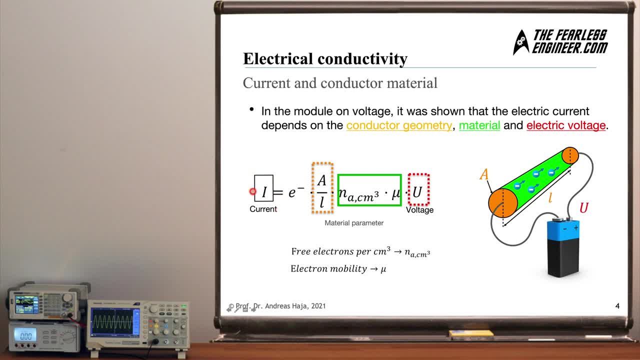 current. But just to recap what you can see here, we have the electric current on the left side, we have the voltage of the battery on the right side and in front of the battery we have those two clusters of parameters. The first is associated to the geometry of the conductor, which is 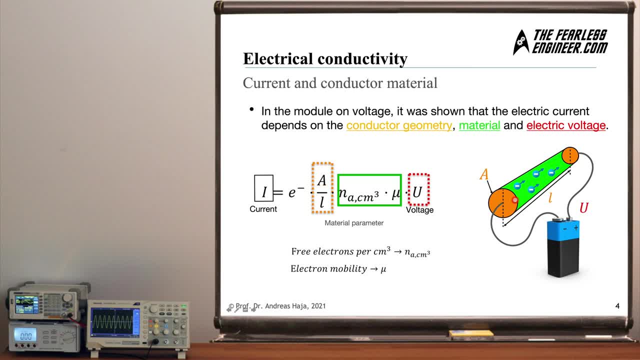 represented by its surface area, the diameter of the cable. you can see here on the right and also the length of this body here And we have the electrons moving through the conductor, driven by the electric field over the length L and the energy. 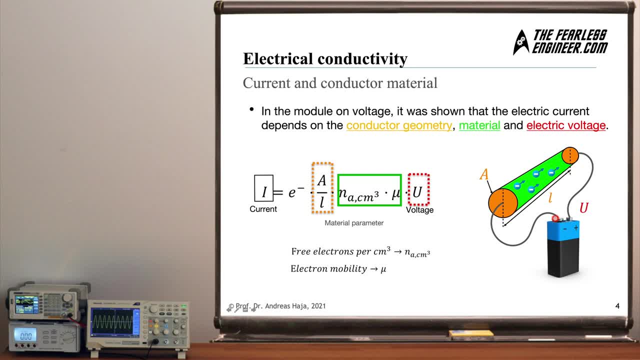 which is transferred to them is taken from the electric field generated by this battery. here And in the green box we have the material dependent parameters, which are the number of electrons in a cubic centimeter of the respective material, for example copper, and also this parameter here is. 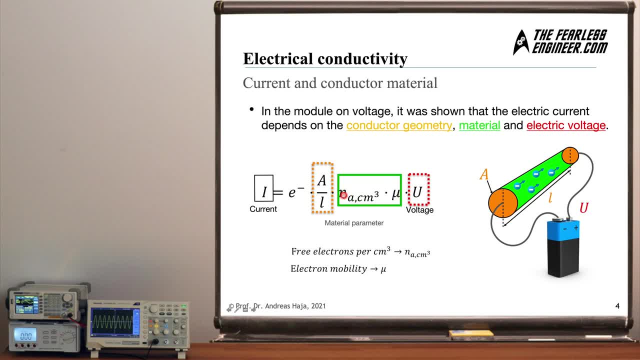 the electron mobility. And, to be more precise, maybe this parameter here is not the number of electrons, but it's the number of free electrons which are free to move under the influence of the electric field. We have already talked about valence electrons when we discussed the structure of atoms. 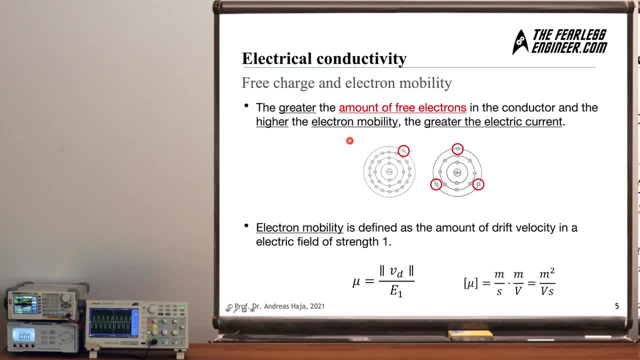 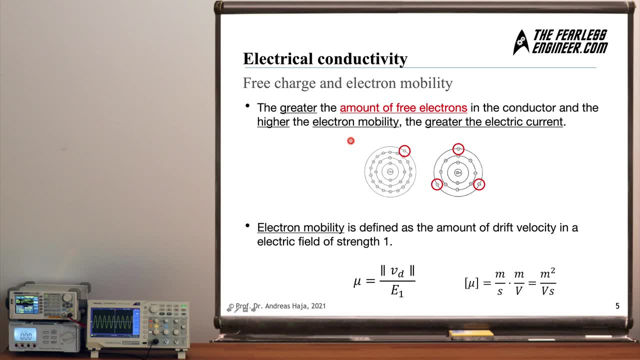 and these are only the free moving electrons. It can easily be understood that the more charges we have which are moving through a cable, let's say the higher, the larger the current which is moving through this cable. So if we succeed in increasing the amount of free electrons in the conductor and also maybe 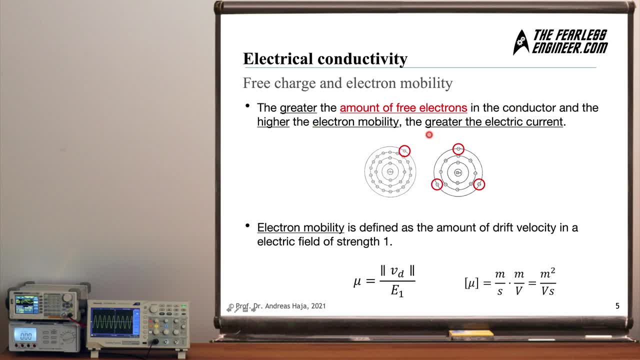 increase the electron mobility, we will be able to increase the amount of current flowing through this conductor. The greater will be the electric current. And here you can see two models of metallic atoms. This is a copper atom with 29 protons in the core and an equal number of. 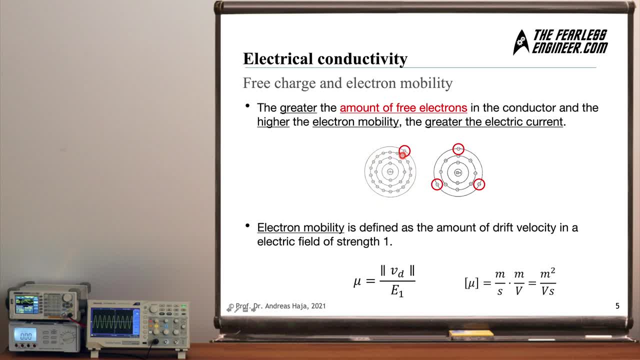 electrons on the various orbits surrounding the core, And the outermost one here in the red circle is called the valence electron, which I already talked about a few minutes ago, And this one is free to move as soon as the copper electrons of the wire arrange themselves in a lateral. 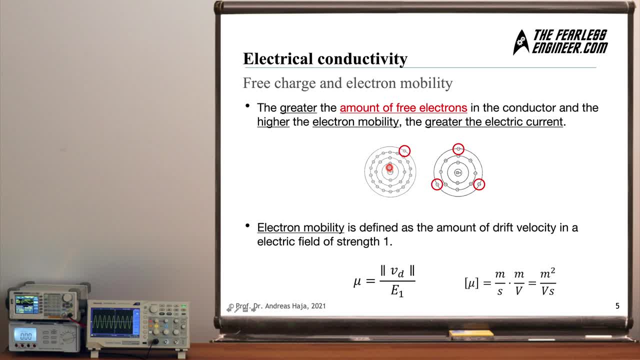 lattice structure And this very dense structure frees up the outermost electrons, the valence electrons. And when we have an aluminum cable, for example, this is an aluminum atom. it has 13 protons in the core and three valence electrons on the outermost shell. Then, per aluminum atom we 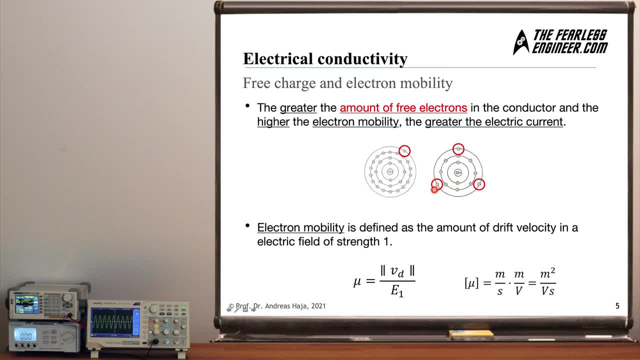 have the number three valence electrons, which are added to the number of free moving charges in this cable. Now the electron mobility is defined as the amount of drift velocity in an electric field with strength one. So we have already talked about drift velocity. If you do not know what this term. 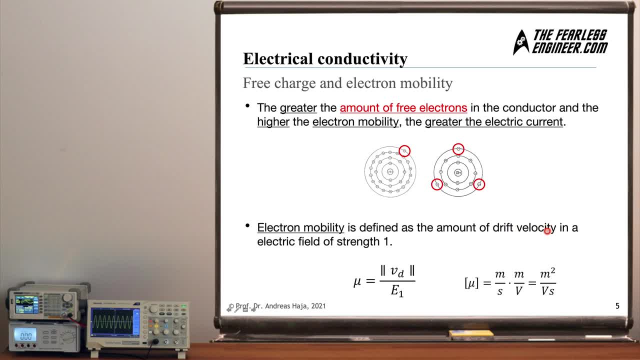 means. I want to refer you to the respective video. And if we observe the drift velocity under the influence of a certain electric field, you will note that there is a relationship, when you recall this video, between the strength of the field and also the electron. 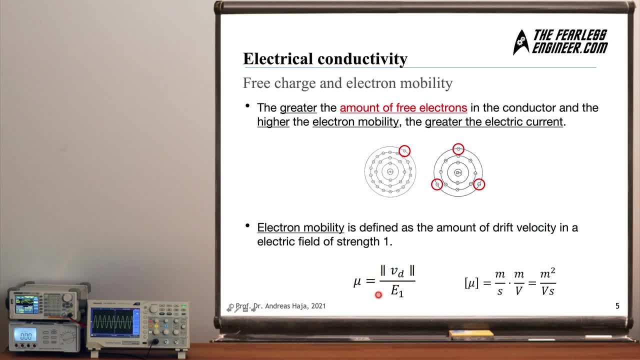 mobility. And now we will rearrange this equation, which you can see here on the bottom left. Usually what we have seen before is drift velocity. Vd equals electron mobility, which is now on the left side, times the electric field strength. And this electron mobility here is defined. 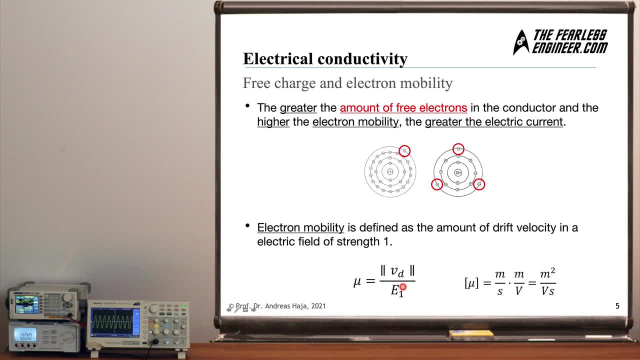 as the drift velocity in a certain material under a very controlled electric field of strength one. So we set this field here to one observe the drift velocity, or record the drift velocity of the electrons moving through the conductor, And this then is the electron mobility, And the unit of the electron mobility is square meters per volt. 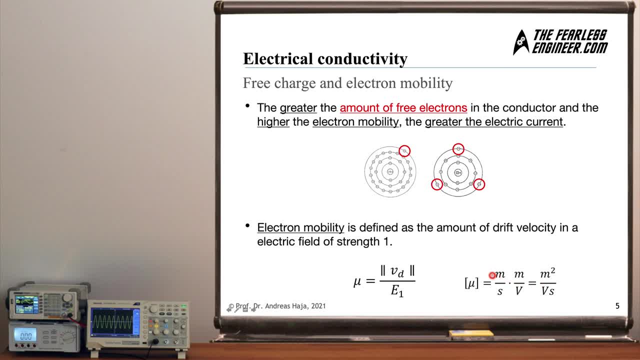 second, And here you can see where this expression comes from. So, meters per second, this is clearly the drift velocity, and volts per meter, This is the unit of the electric field, which is now inverse because it's in the denominator, And, in summary, we get square meters. 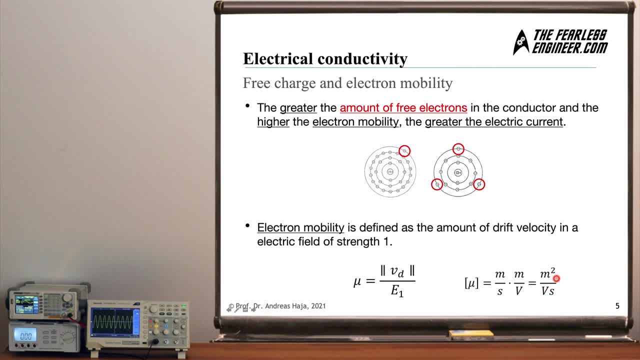 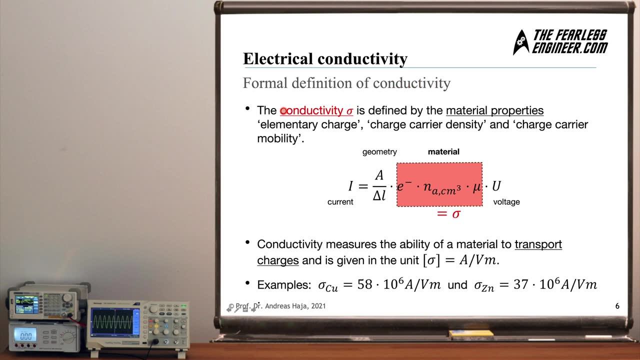 divided by volts. That's the unit of the electron mobility, And from the units here it becomes clear that this is the definition behind electron mobility. Now let's look at a formal definition of electric conductivity. The electric conductivity gets the letter sigma, And sigma is defined by the material properties, the elementary. 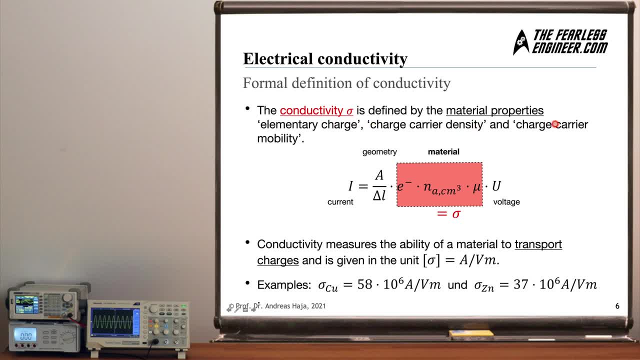 charge, the charge carrier density and the charge carrier mobility, And all the material parameters which I just mentioned are depicted here inside this red box. We have already discussed this equation before. Now we are focusing only on the material dependent parameters And this product of 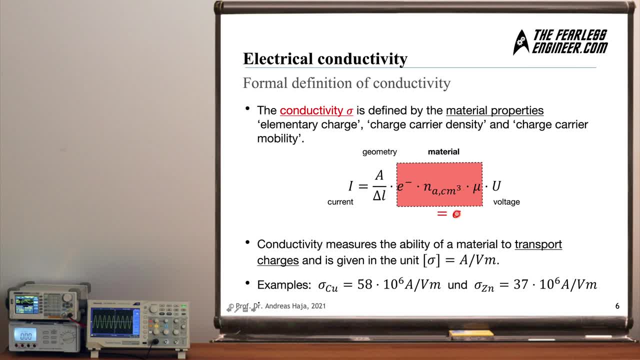 these three parameters is what we term conductivity sigma And conductivity measures: the ability of a material to transport a certain number of charges, free charges, through a conductor under the influence of an applied voltage, And it's given in this unit here, amps per volt meter. 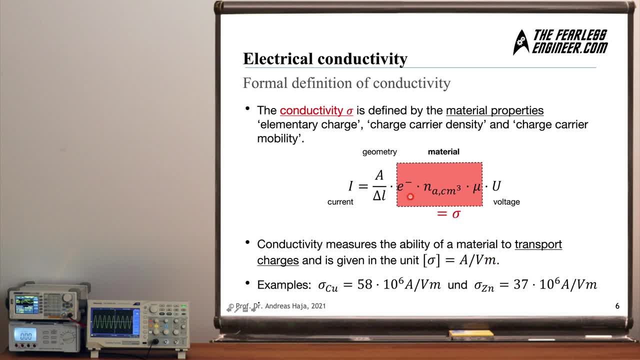 And in order to understand where this unit comes from, you only need to look at the units behind these three parameters here, and then you will arrive at this definition here. Let's look at two examples. The conductivity of copper is 58 times 10 to the 6 amps per volt meter. 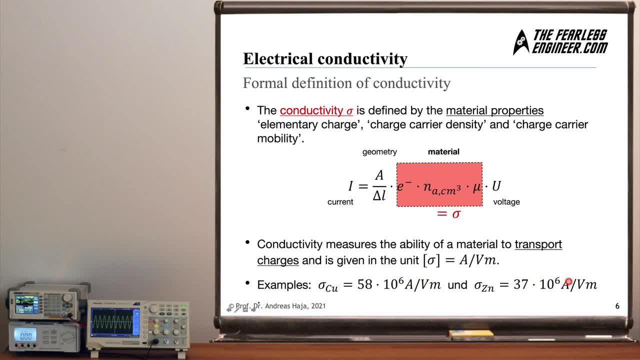 and zinc is only 37 times 10 to the 6 amps per volt meter. So from these two numbers you can see that copper is a much better conductor than zinc, for example. Now, the major aim of this video was to build a bridge between these two units here. 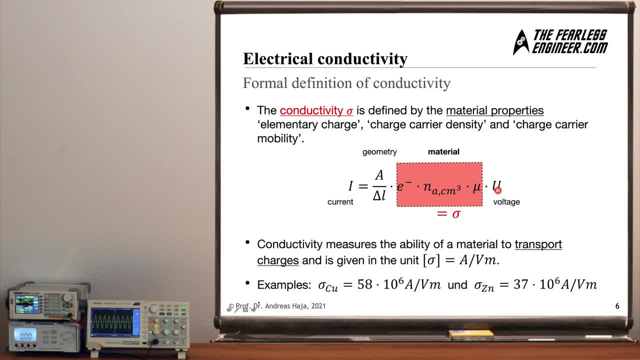 current on the left side and voltage on the right side. And in the long run, we want to get to Ohm's law, which introduces the concept of resistance in order to relate the two current and voltage, And on our way there, to this concept of resistance. 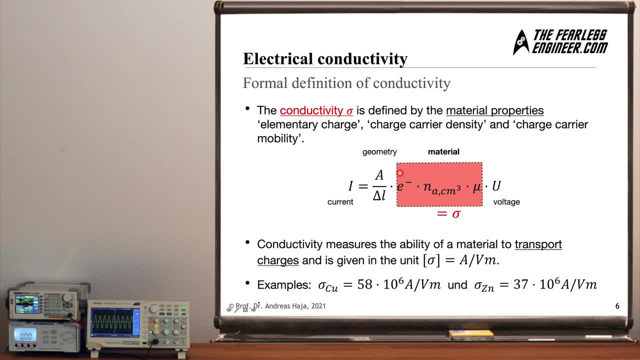 we now introduce the concept of conductivity, which summarizes some of the parameters from this rather lengthy equation to make it easier to glimpse the resistance which already is hidden in this conglomerate of parameters. It's defined by the conductivity, it's defined by the cross-section area of the conductor we are looking at.